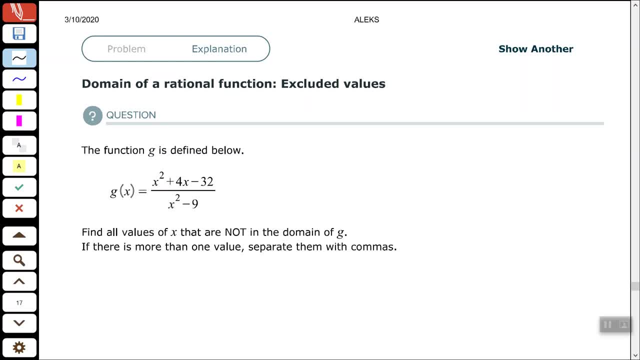 Hey, hey, good people. Arthur Morris here, Hope all is well. In this video we're going to look at the domain of a rational function. We want to find the excluded values. That's what we want to do. So it says the function g is defined at below. g of x equals x squared plus 4x minus 32, over x. 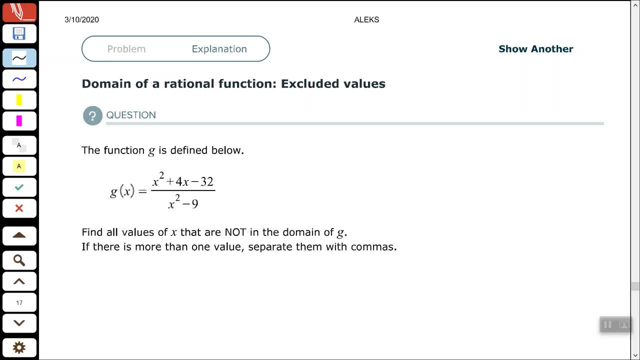 squared minus 9.. So we're not simplifying anything. We want to find all the values of x that are not in our domain of g. So the best way to do this: look at our denominator, take our denominator, set it equal to zero and find out what makes our denominator equal zero. Okay, so our excluded 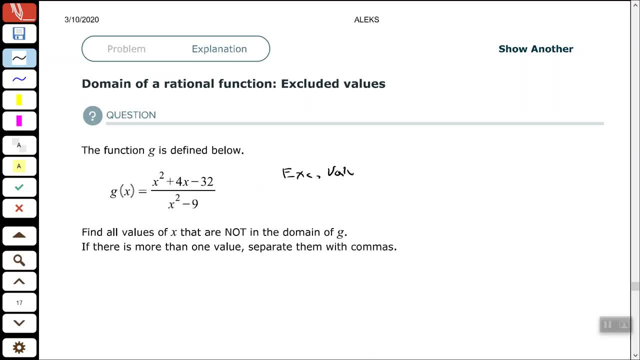 values. Our denominator has the variable of x squared minus 9, variable expression of x squared minus 9.. So I'm going to take that expression, Set it equal to zero And then I'm going to solve. So a couple of ways you can do this. 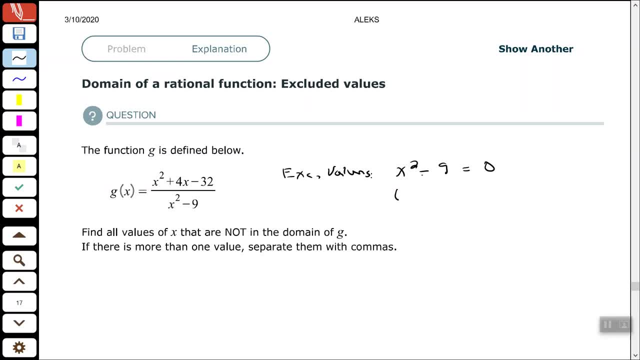 Let's go ahead and use factoring, since that's what we've been using. So if we factor x squared minus 9, that's using the rule a squared minus b squared, which equals a plus b times a minus b, So that factors out to be x plus 3 times x minus 3.. 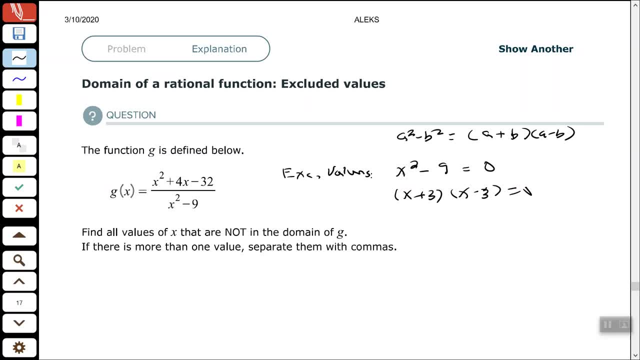 And then remember, when we have two factors like that set equal to zero, we split it up, set each factor equal to zero and solve So subtract 3.. So one of the excluded values is negative, 3. Add 3. The other excluded value is positive, 3.. 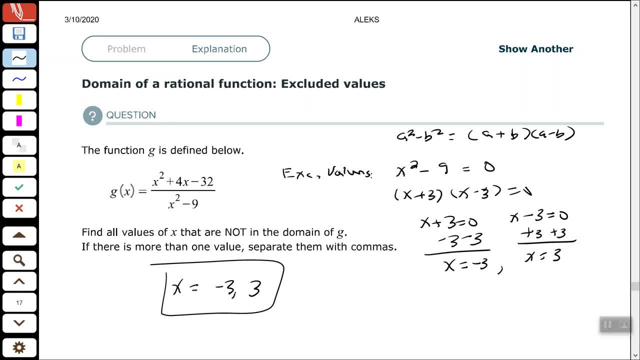 So my excluded values are negative 3 and 3.. So again, yes, those are exclusive ones. So if we look at this denominator equal negative 3, what do I get? I get x times u square negative 4.. And then here, if we look at these educators, less than negative 3,, I get perfect 0.. 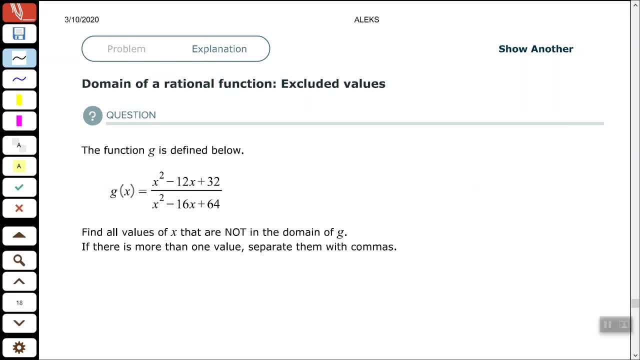 Even though I built this number, I don't want to gegangen be more than negative 3, because y equal to negative 3.. Okay, So let's do it again. If we look at this denominator B that are not in the domain of G, So we want to look at our denominator set it.